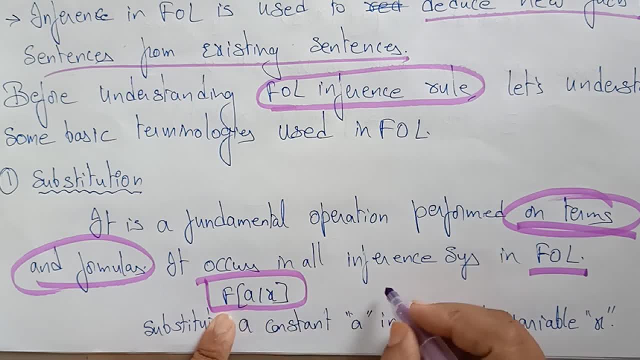 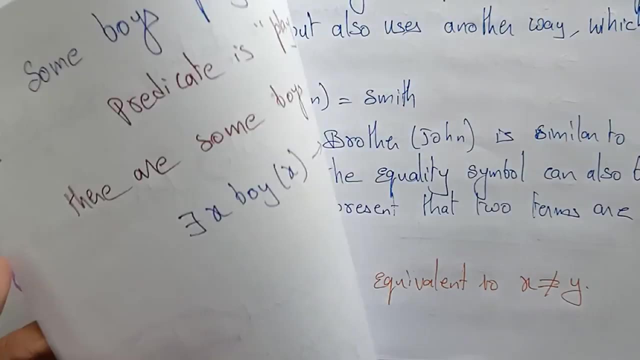 variable in x. that variable you have to write here. Suppose I want to substitute b by x, means in place of x I want to substitute b. So this is the first order inferences in the first order logic. The first thing is a substitution. Now let's see the another thing, that is, the equality. 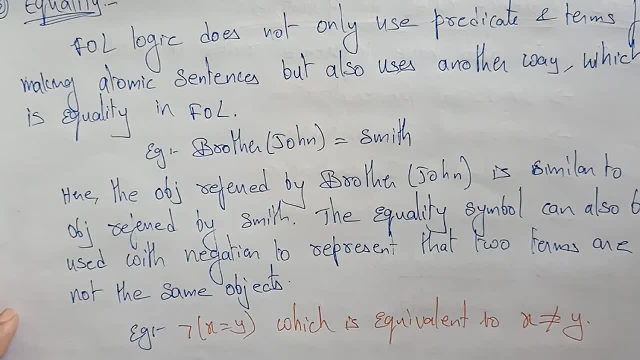 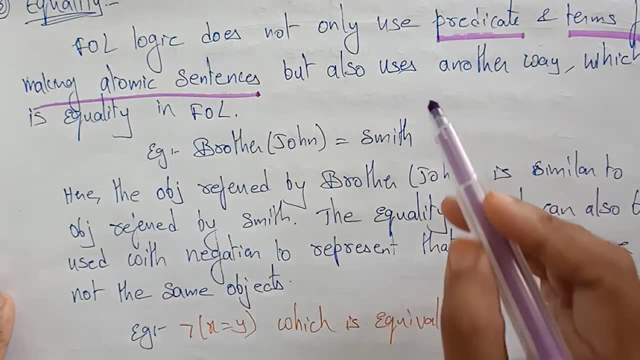 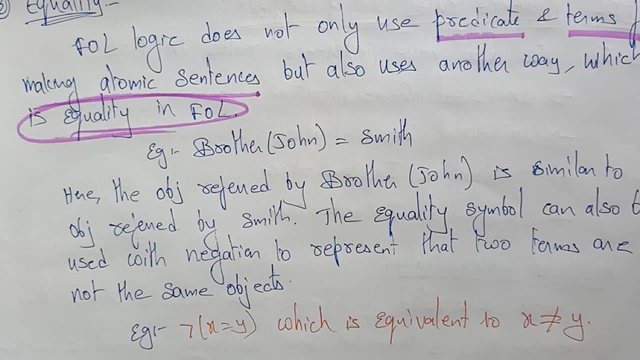 Equality. The another term in this here is the equality. The first order logic does not only use a predicate and terms for making atomic sentence, but also uses another way, which is the equality in the first order logic. So far you had seen the predicates and the terms that use making atomic sentence, The atomic statement. 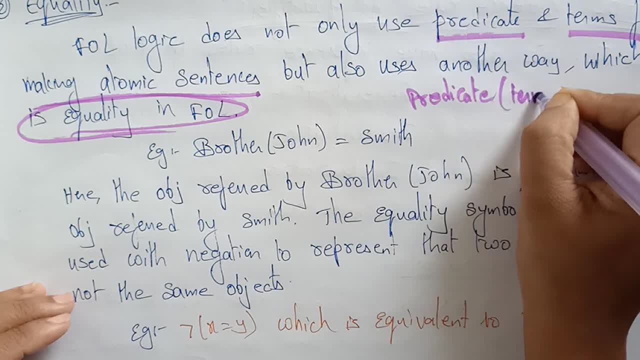 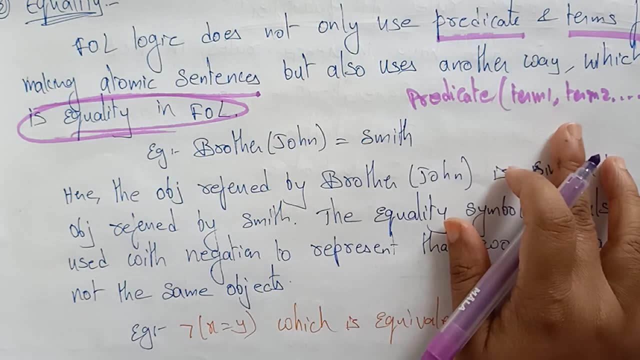 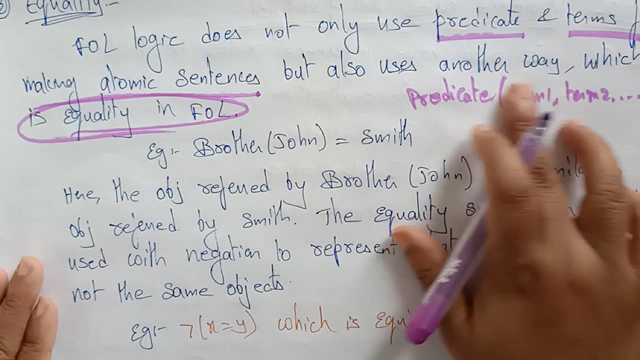 is represented as predicate And here there are some terms: term one, term two, like that. Okay, so far you have seen this atomic statement here like this, In the first order logic. it not only contains atomic statements, but also it uses in another way 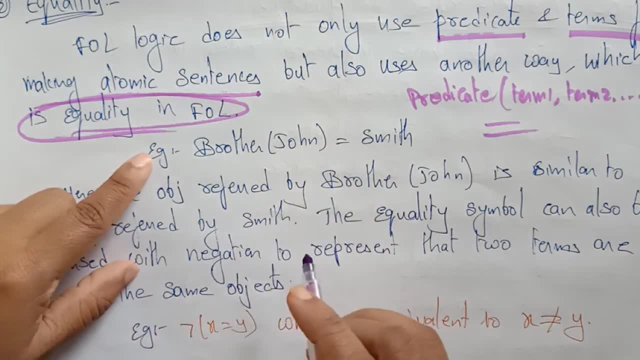 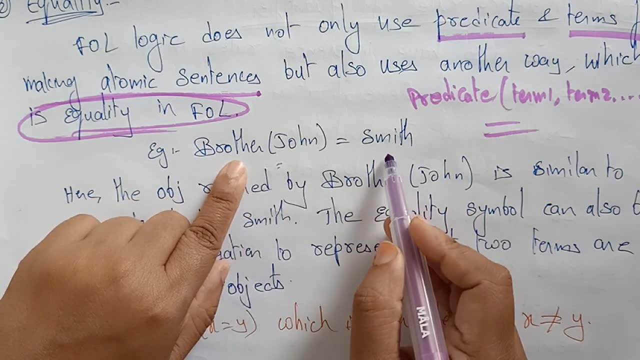 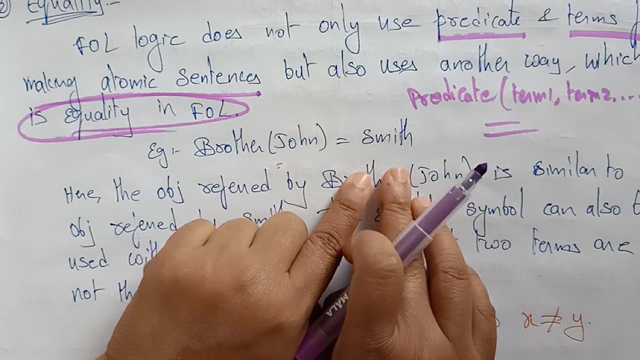 that is the equality, This is the equal symbol. The example for here is: suppose the brother John is equal to Smith Means the John's brother is a Smith. So did you observe here, Smith is the brother of John and John is the brother of the Smith. So in that cases you have. 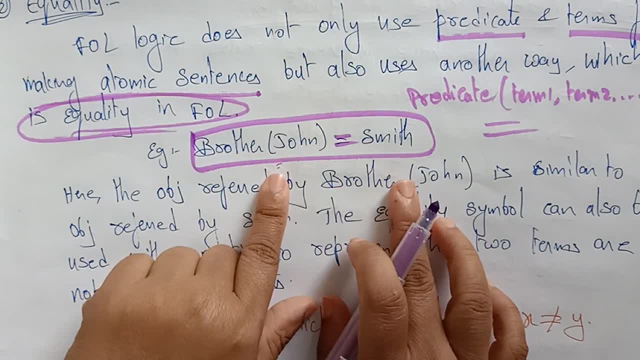 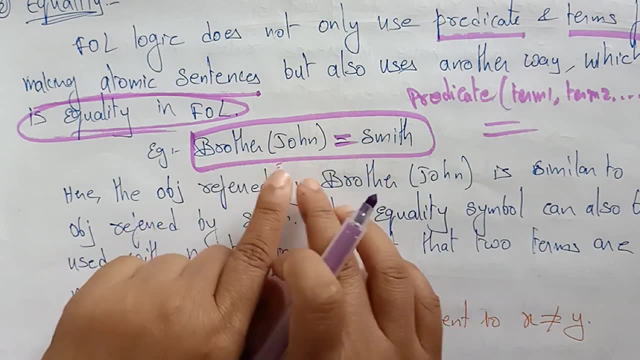 to use a symbol equality. So in that case you have to use a symbol equality. So in that case you have to use a symbol equality, Because John is the brother of Smith and the Smith is also a brother Whenever he is. brother means obviously he is also brother to his right. So here the 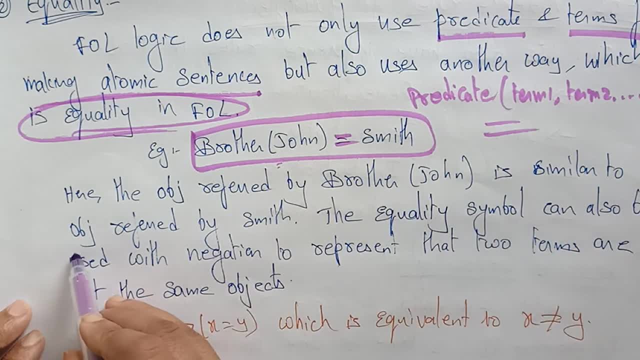 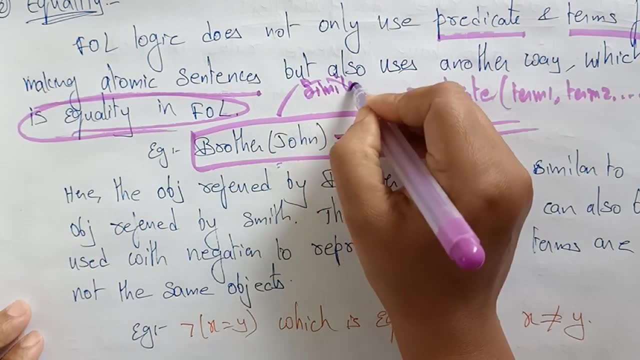 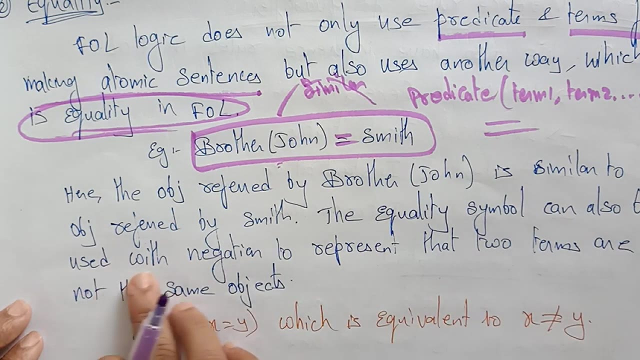 object referred by brother John is similar to the object referred by the Smith. So this is: both are the similar. Because the object referred by brother John is similar to the object referred by the Smith, The equality symbol can also be used with the negation to represent the two terms are not the. 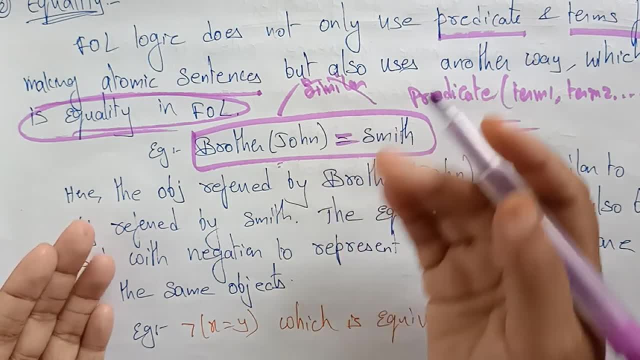 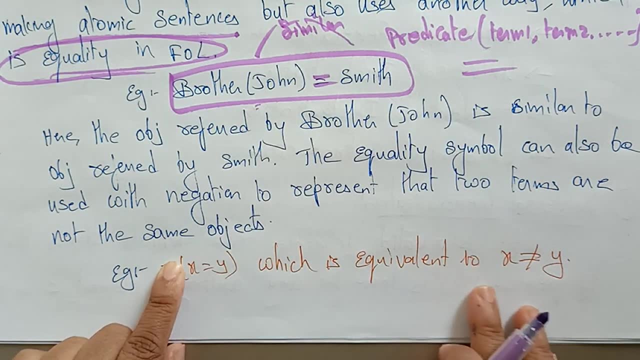 same object. Not only this equality symbol, you can use for the negation also How it is. let's see Negate: x is equal to y. That means it is equivalent to that. x is not equal to y. Both are the same. 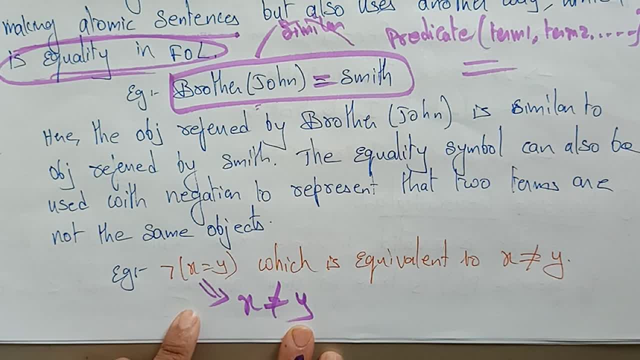 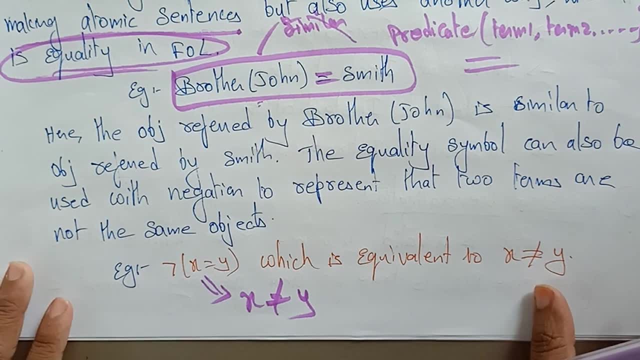 You can represent this statement as this, like also like this: X is equal to y means whenever you use the negate operation means x is not equal to y. So these are the basic terminologies that you use in the inferences in the first order logic. Thank you.